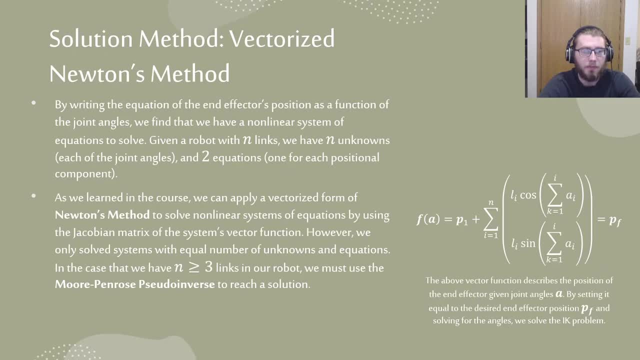 2D space, there are two positional components. So, as we learned in this course, we can apply a vectorized form of Newton's method to solve nonlinear systems of equations by using the Jacobian matrix of the system's vector function during the Newton's method update step. 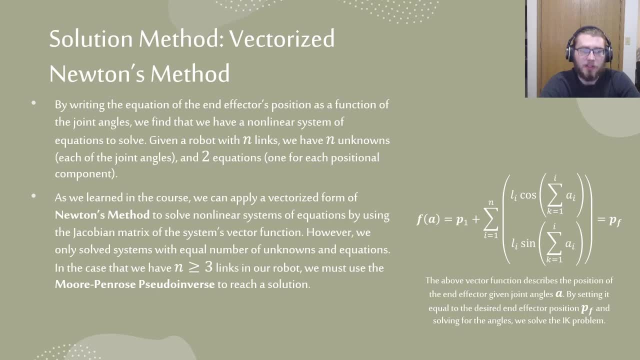 However, we only ever solved systems of equations with equal number of unknowns and equations. This is because whenever we have equal number of unknowns and equations, the vector function in matrix form is square and thus invertible, so we can solve for the increment during the update step quite easily. However, in the case 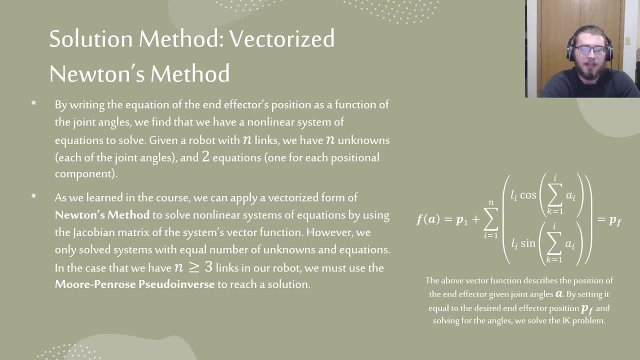 that we have n greater than or equal to 3 links in our robot. the Jacobian matrix is non-square, so we must use what's called the Mohr-Pinrow pseudo-inverse for the method to converge properly. A little bit more about the Mohr-Pinrow pseudo-inverse and why it's needed. 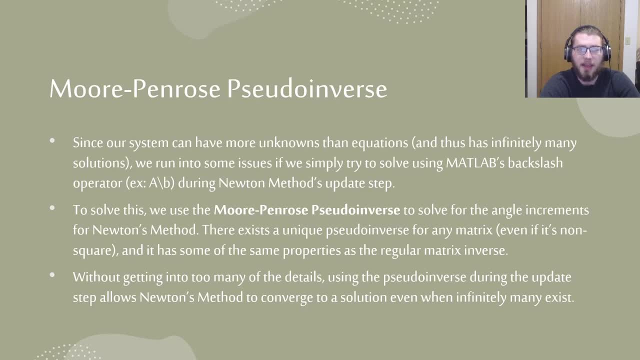 So, since our system can have more unknowns than equations, it actually has infinitely many solutions. in many cases, We run into some issues when trying to use MATLAB's backslash operator during the Newton's method update step, but this is solved by using the Mohr-Pinrow pseudo-inverse. 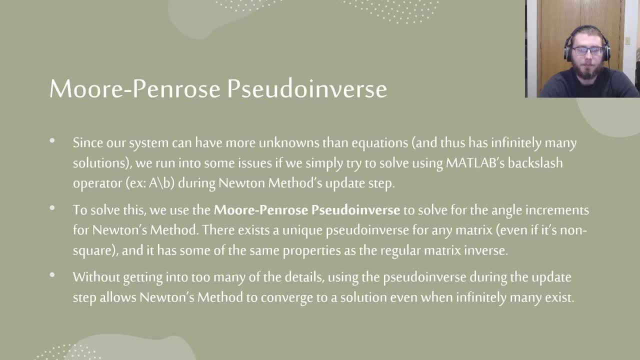 to solve for the angle increment during the update step instead. So, without getting into too much detail about what the pseudo-inverse is, just know that for any matrix there exists a pseudo-inverse of that matrix that is unique and it has many of the same properties as the regular inverse, but not quite all of them. 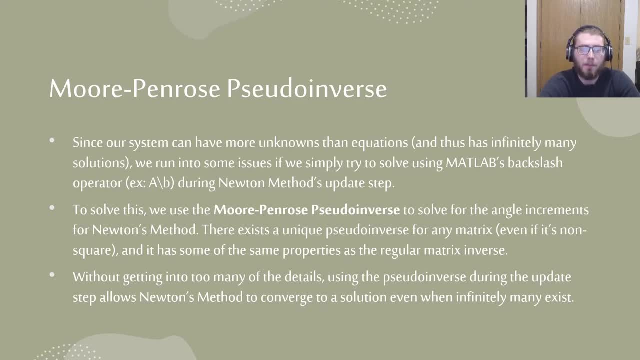 but it also has some more properties that are also useful, And whenever we use the pseudo-inverse to solve for the angle increment during the update step, it does allow Newton's method to converge, whereas it did not with just MATLAB's default backslash operator for solving the linear system. 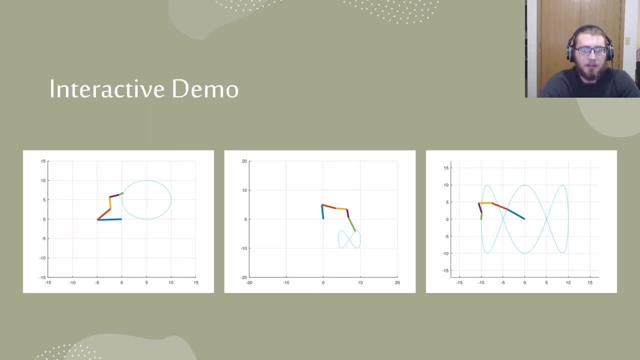 during the update step. So now I'm going to show an interactive demo of my results and show that the solver is indeed solving inverse kinematics problem. What you'll see is a robot positioned in a 2D plane, where the base of the robot is positioned at the origin, and we've plotted 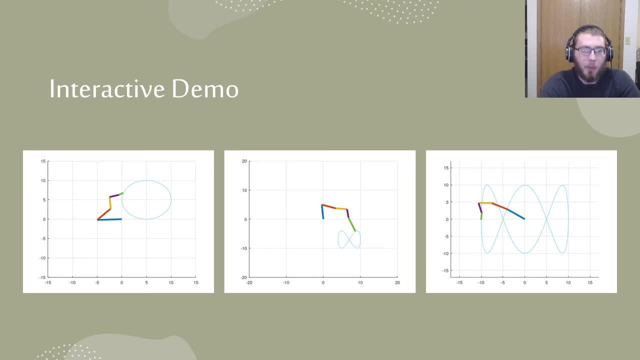 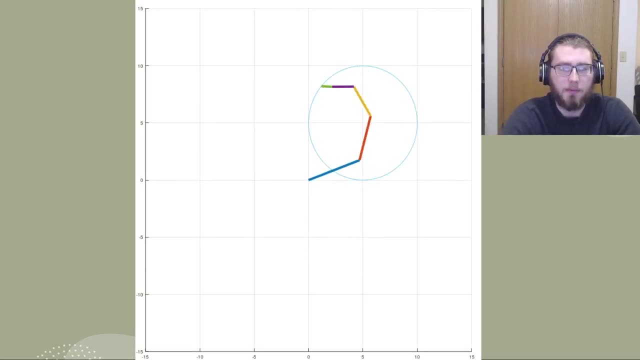 a function in the plane and we're going to have the robot actually trace this function over time. So you should see now an interactive demo. The robotic arm is tracing a circle in the plane and you can see over time it does keep tracing it and what's happening is that each update step 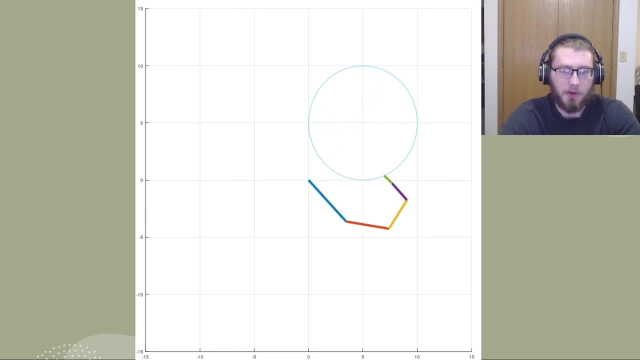 we're calculating the next position along the parametric function, which is in this case a circle, and we're having the solver actually solve inverse kinematics, such that the robotic arm puts an end effector at that location. So now we'll take a look at another function. 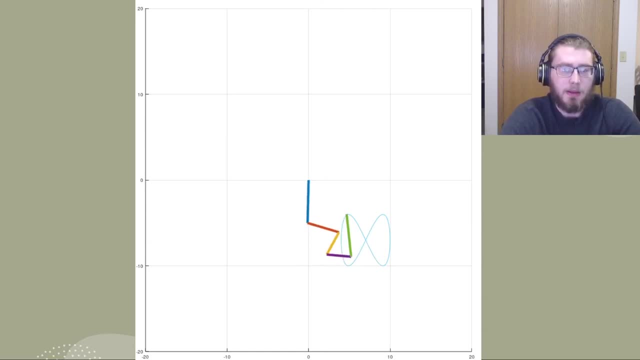 So now here's a slightly more complex function. We've also changed the configuration of the robotic arm. just to show that the solver actually works for any configuration In this case, I just changed the last link. I made it a little bit longer. You can see it's. 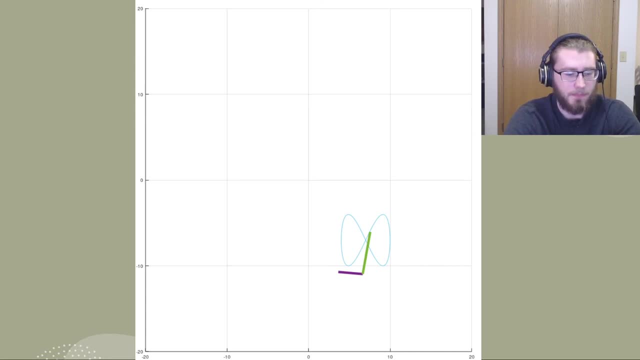 tracing just fine, and we'll show another one. So here's another function that's being traced. It's a little bit more complex And it's also moving faster, and you can see that the robotic arm traces it just fine. So this is a nice interactive demo showing that the solution that I wrote does work.